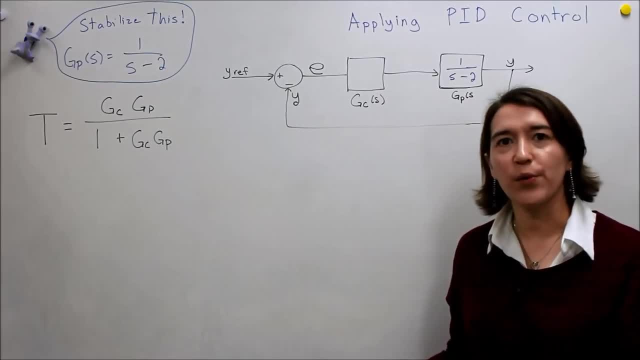 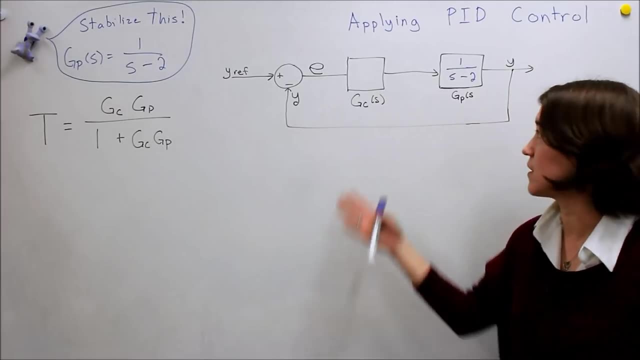 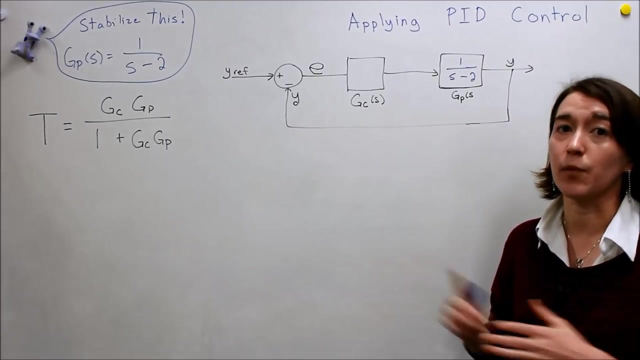 to stabilize it. So well, how are we going to do that? The system is what it is. We can't really change that. What we can change as designers is the controller. So we know that a proportional control did not work, so why don't we just look at PID- proportional integral derivative control? 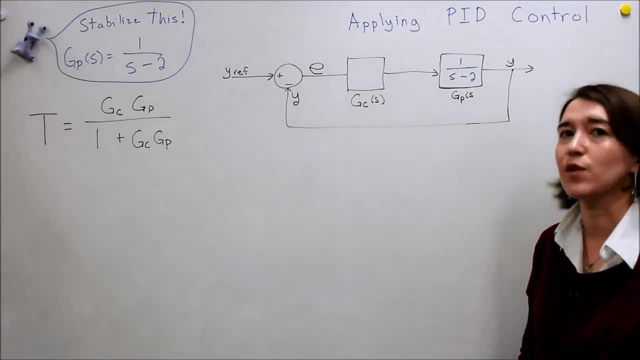 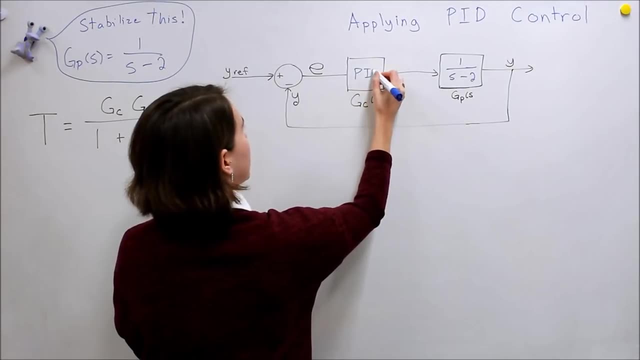 and see if we can apply that to the system and see if we can stabilize it. So to do that, we'll start with I'll just write PID in here. Now we have to write the equation for that. So let's write the equation for that right here. 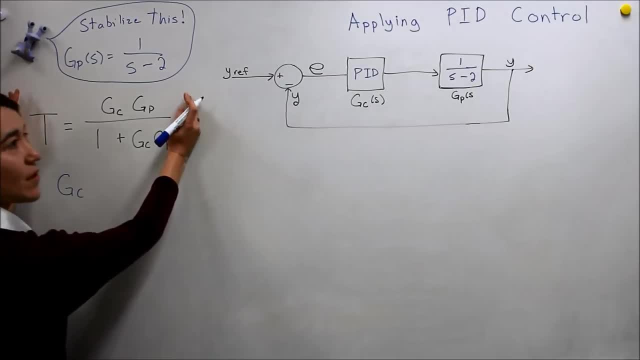 So this is going to be GC and this is our closed loop transfer function, if you remember. So we need to write the equation that we're going to put into here for the GC. okay, So if you remember the different parts of PID, you just kind of add the three different parts together. 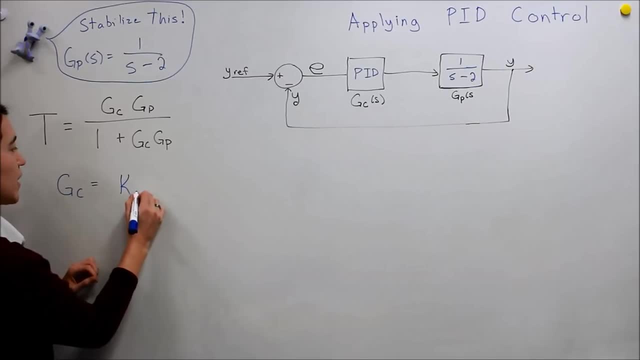 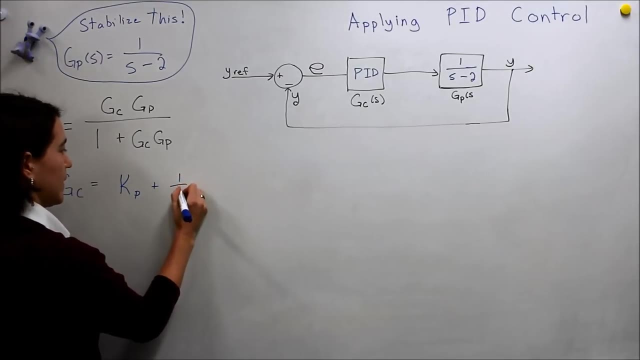 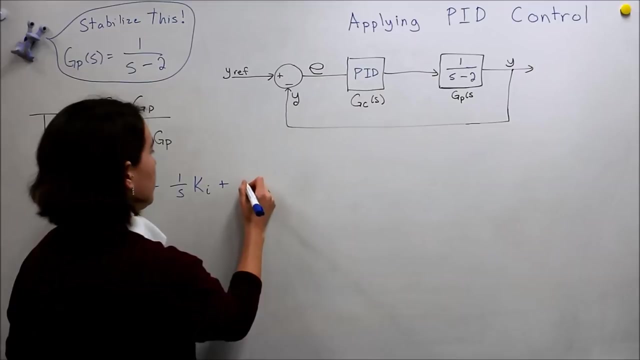 So P would be some constant and we're going to call a little p there for proportional constant. Then we have integral, so 1 over s, And then we have a coefficient. so we have k and we're going to call it i for integral, And then we have the derivative control. so we have 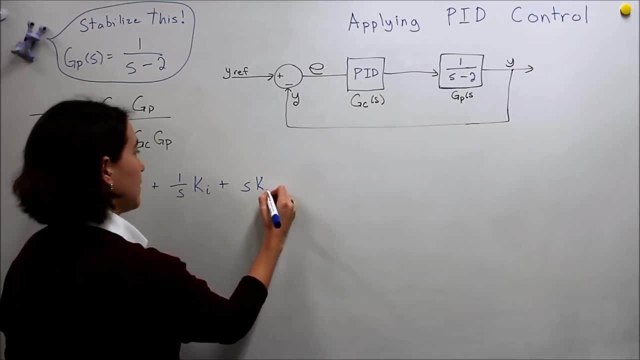 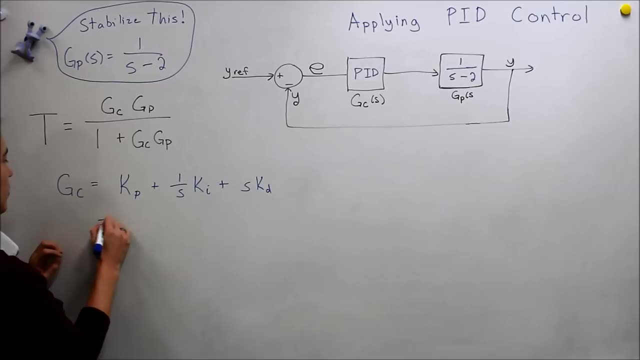 a derivative, and then we have- we're going to call it kd for derivative, And so let's put this into just one, combine this into one equation or one fraction, And if you multiply this by s over s, multiply this by s over s, we will get the expression. 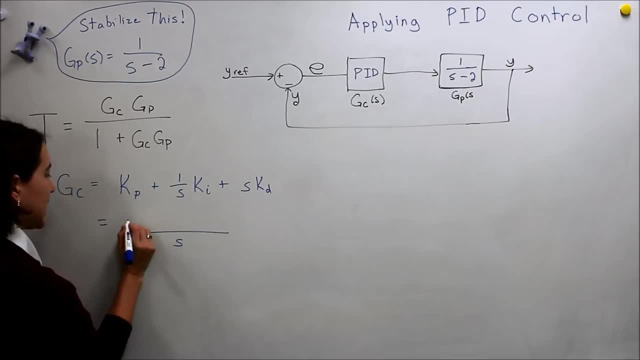 And I'm going to just read this: Let's reorder in here so we would get kd s squared plus this kp times s and then plus just a ki here. So this would be the fraction form of our controller, the PID controller. okay, 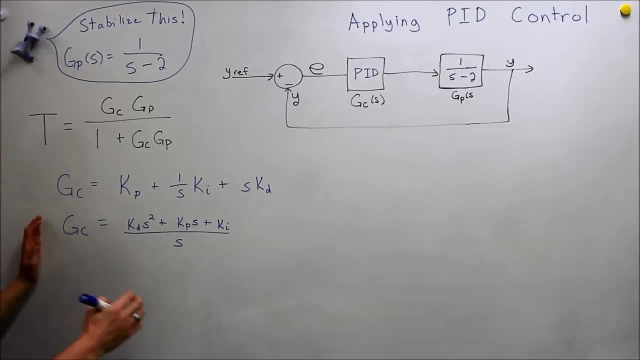 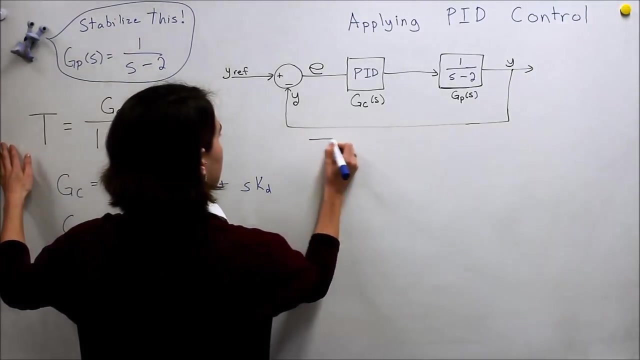 So we have our two expressions here. We know GC, we already know GP, and so we're going to put it into our closed loop function and see what our output, our total closed loop transfer function, will look like. So we'll do that over here. 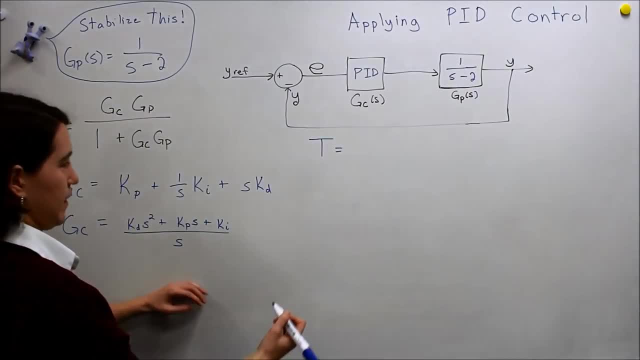 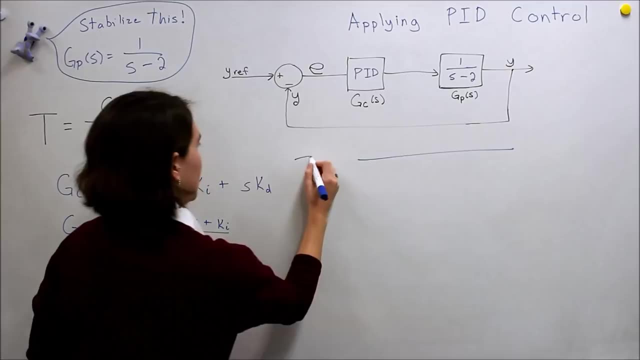 So t equals. okay, so this is going to get a little bit exciting here, Okay, so I'm going to move this down actually. So we're going to go: t equals, so we have this whole expression right. so we have kds. 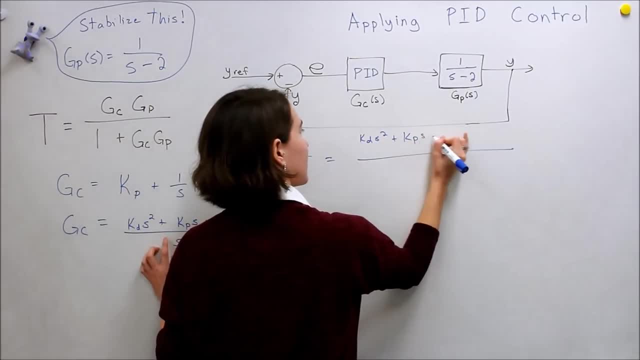 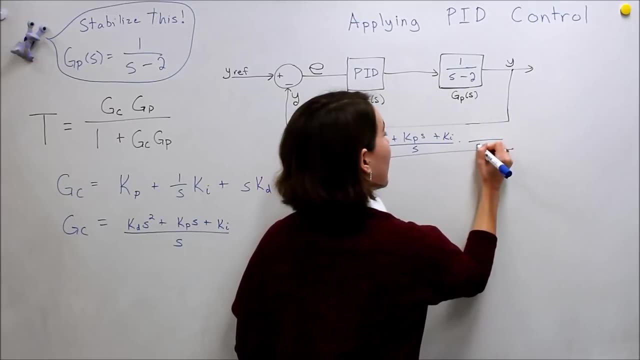 squared plus kps, plus kd. Okay, All right, So we have: t equals s ki. This is all over s. And then we have this function. so we have multiplied by s minus 2 over 1.. And then we have that same exact thing. 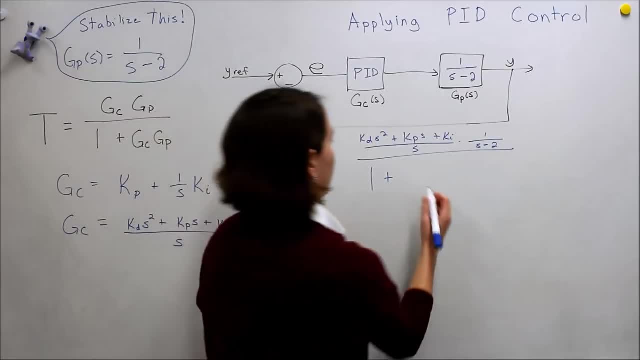 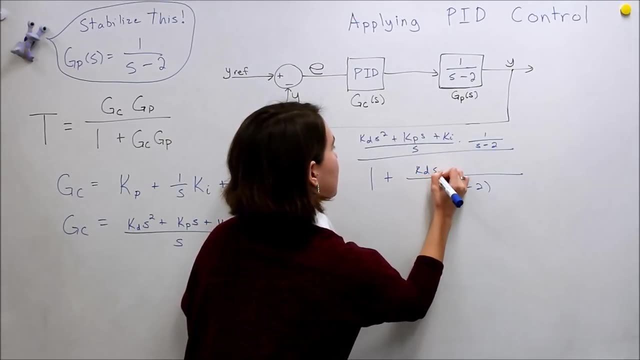 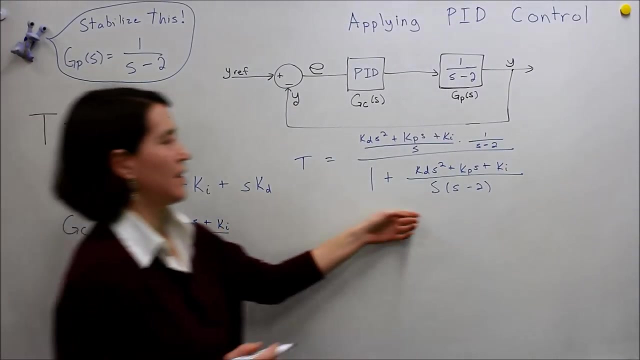 The numerator denominator is 1 plus that whole thing, So we'll just write it here. So we get s s minus 2, this guy on the top kds squared kps plus ki. All right, We don't like these s's in the fractions, so we're going to multiply both sides by s. 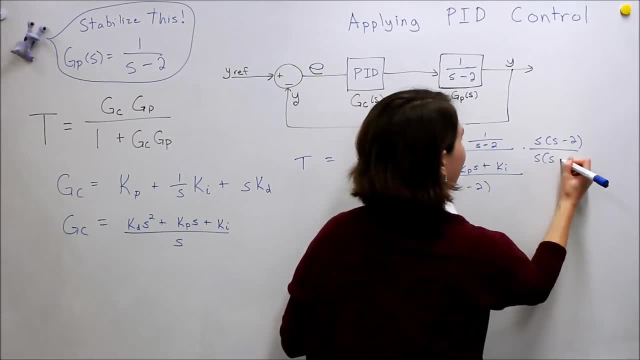 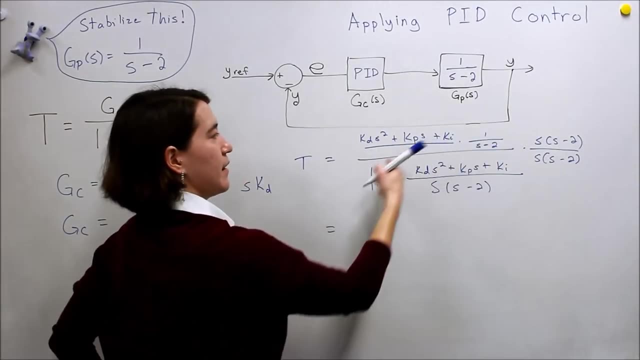 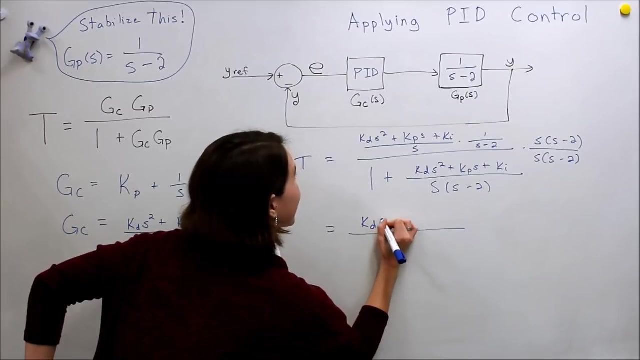 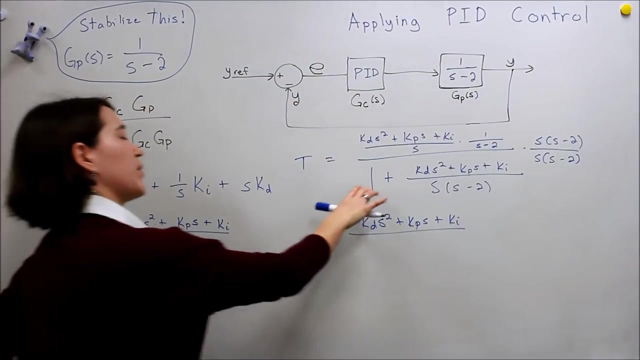 s minus 2, both top and bottom. Okay, that will. let's evaluate that right here. So that gets rid of the numerator denominator here. so we'll just have the total numerator. we'll just have k d s squared plus k p s plus k i, and then we'll do the same multiplication. 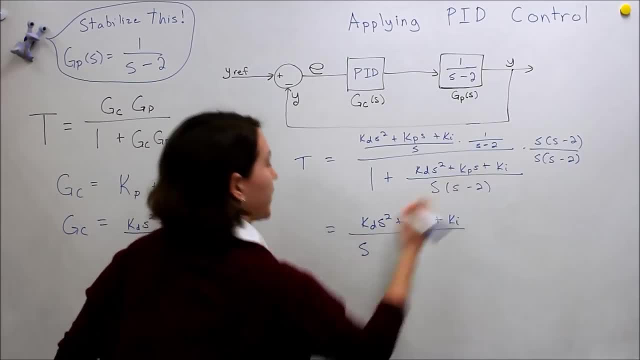 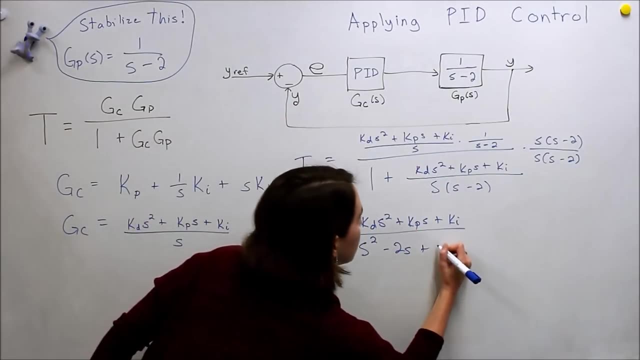 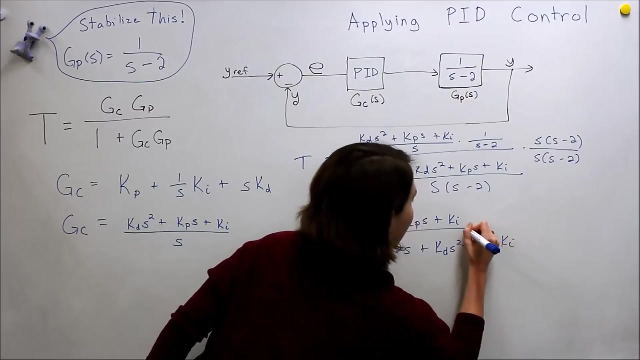 here and we get s. we're going to just multiply it out: s squared minus 2, s plus just this expression. So k d, s squared plus k, p, s plus k i. Alright, And now let's in the denominator, let's bring common terms together. 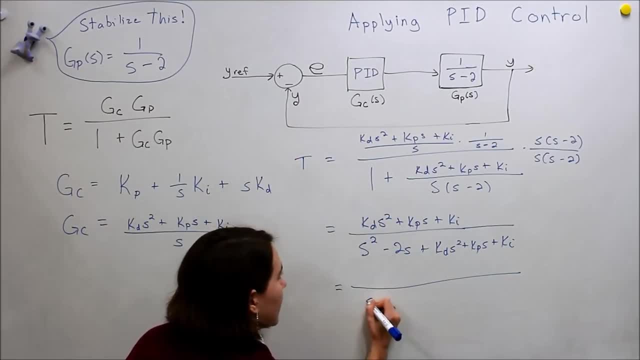 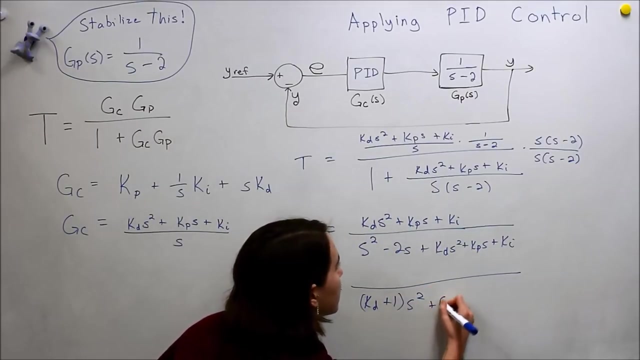 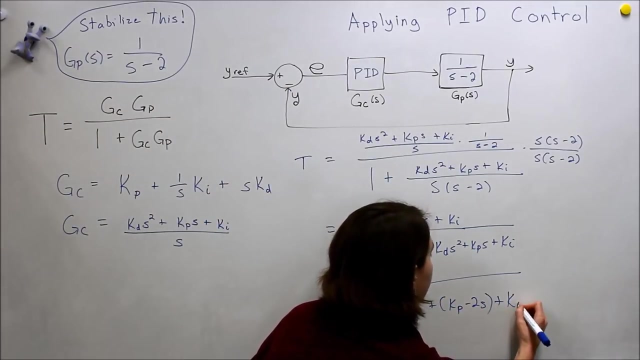 So we'll end up with s. well, k d plus 1 s squared. and then let's look at the s's. So we have these two values here, So it's k p minus 2 s, and then we have a k i plus k i. 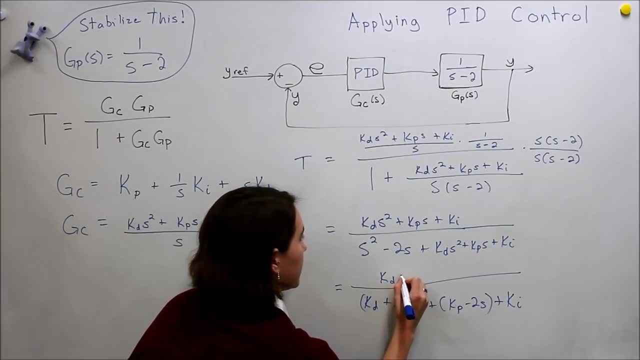 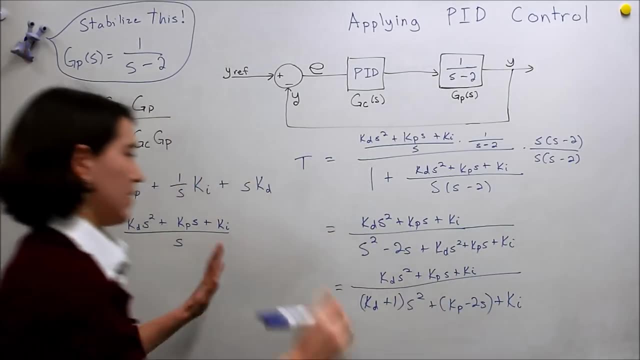 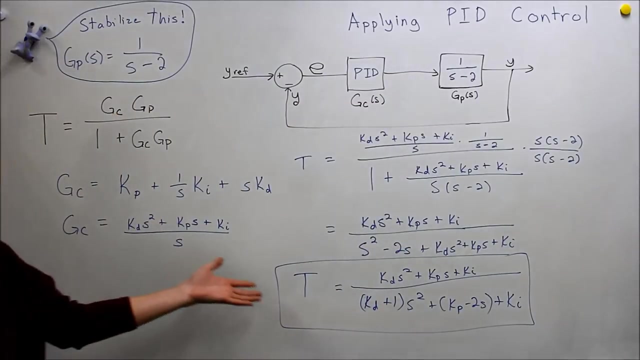 And the numerator here will be the same: k d s squared plus k p s plus k i. Okay, so here is our overall transfer function implementing PID control. This is before we had not chosen the values of our coefficients, so this was what once. 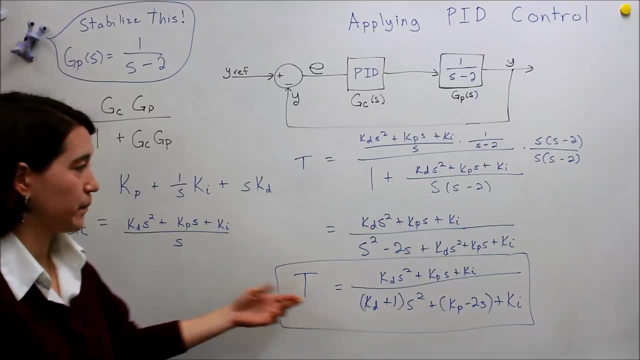 we picked those values, we would plug it in here and this would be our transfer function. Well, what are we going to do? Well, we're going to plug it in here and this would be our transfer function. Well, what are we going to do? 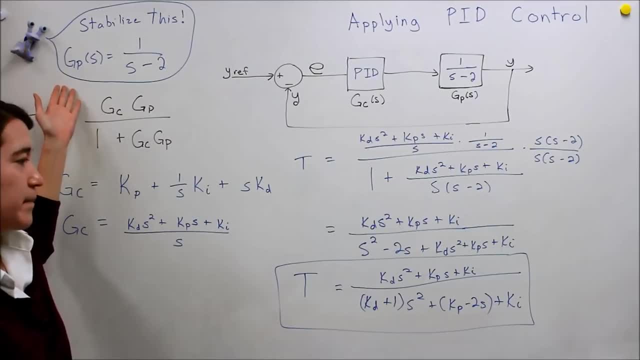 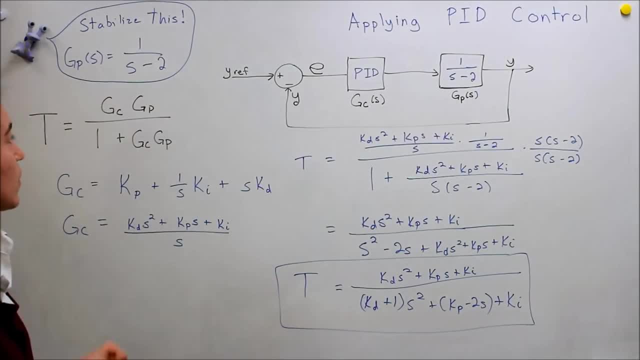 So we're going to pick them to be in the left half plane because we know that's stable. So let's, for example, say we want our poles at negative 1.. So negative 1, negative 1.. Because this is a second order, so we can pick the two poles. we want them to be negative. 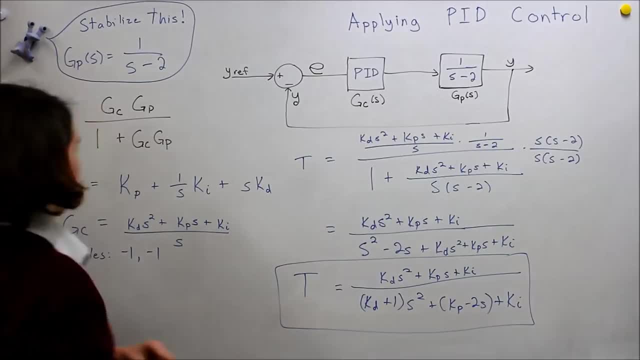 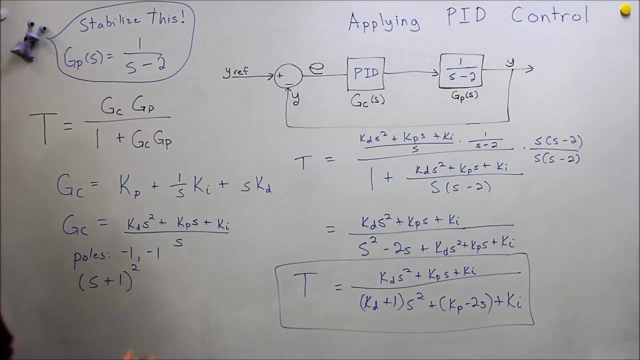 1, negative 1.. Let's see if we can make that happen. So if we did two poles at negative 1, we would have s plus 1 squared. That's what we want our denominator to look like. And if we multiply that all out, we would get s squared plus 2s plus 1.. 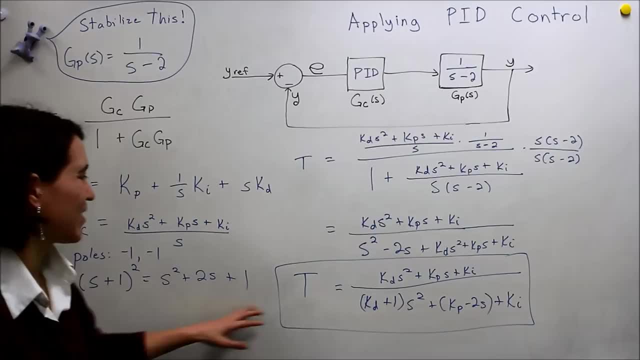 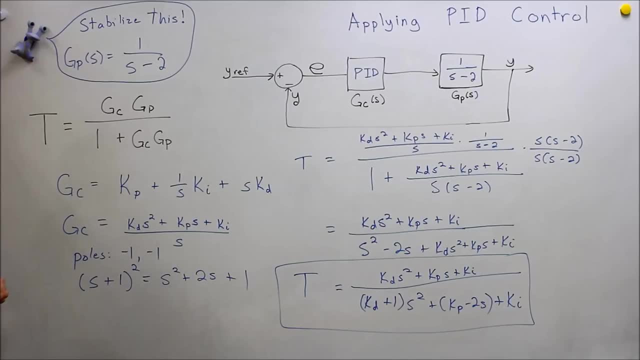 So all we have to do now- hopefully to achieve that- is to make these look the same. So not too bad, Let's see if we can do it. I'm running out of board space. We're going to do this. We're going to start writing it up here. 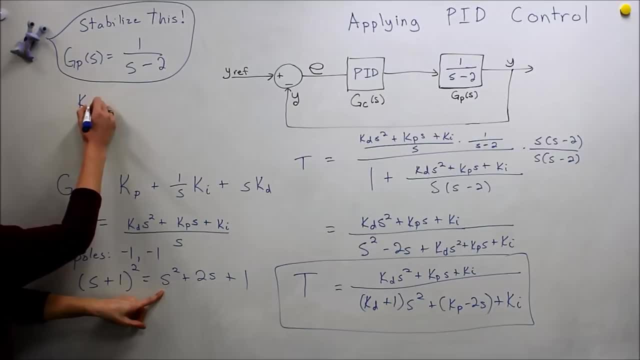 So all we need to do is make kd plus 1 equal to this coefficient, which is 1.. And then we need this kp minus 2, to be equal to 2.. And then we need ki to be equal to 1.. 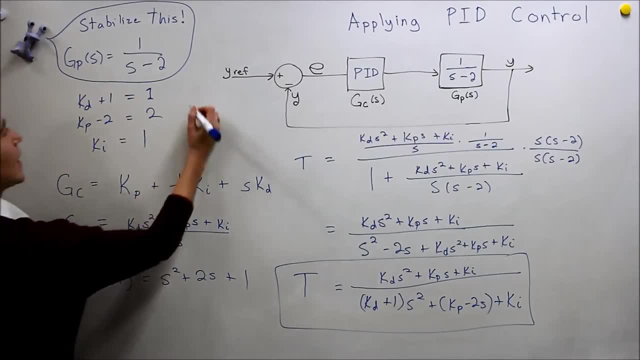 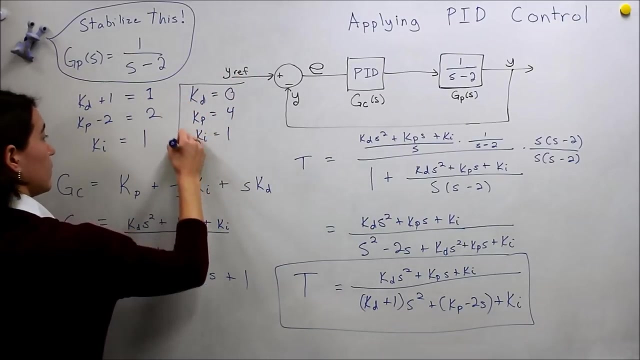 So if we just do these calculations, we'll see that. So kd equal to 0 actually will satisfy this equation, kp equal to a positive 4. And then ki equal to 1 will put the two poles at negative 1 and negative 1, which means 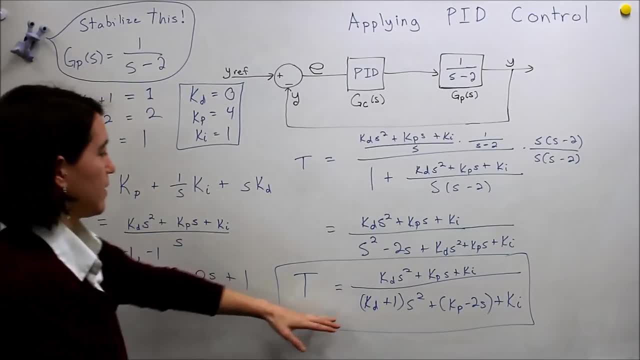 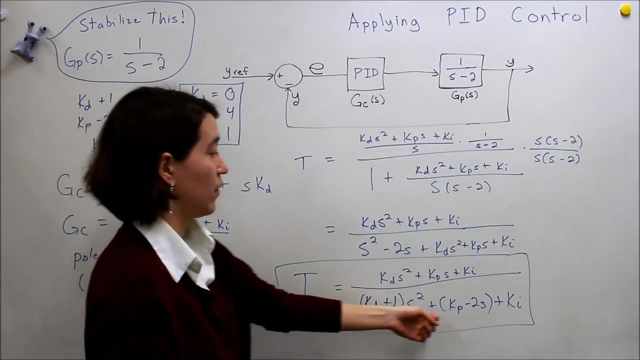 that our system will be stable. So, going through this process, and if, in this case, we just picked poles, instead we want these specific poles. So this is the same as in the previous equation. This is the same as the previous equation. choose these coefficients to achieve that. 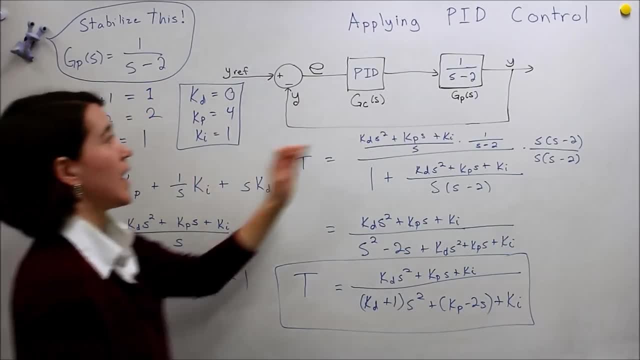 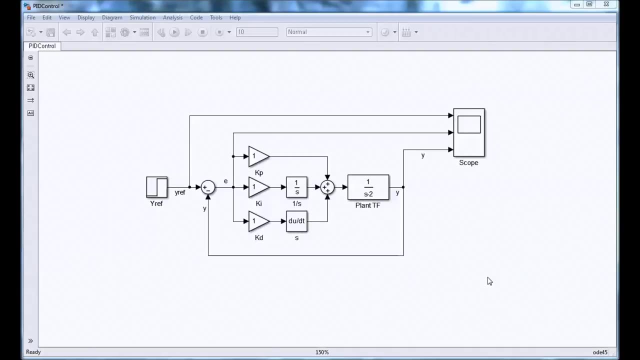 So if we put in these coefficients we should see a stabilized output here. So let's look at that in MATLAB real quick and just confirm our findings Here. we have our system in MATLAB Simulink and we have our plant and this is a the block or multiple blocks to make up the control system. 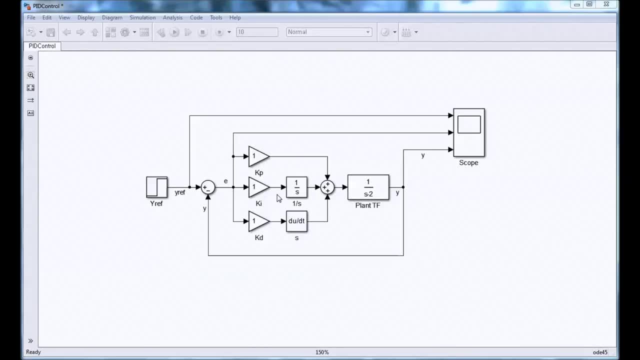 So here we have the proportional control, integral control and the derivative control here, And we want to now implement the correct PID control to make our system stable. So just to show that these values are actually important. first I just started out with ones, because when you put them down in Simulink they just start. 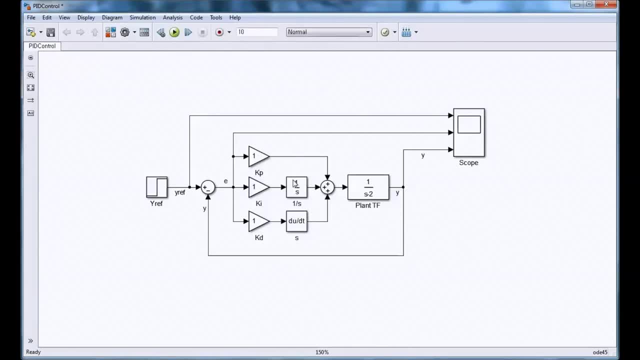 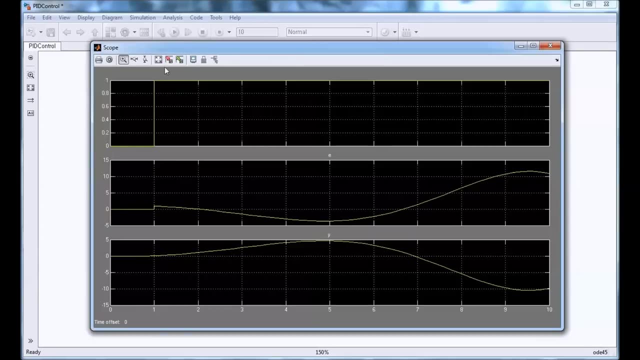 as one. So let's just see if, for example, this- just implementing some PID and picking some values- if that will make it stable. So we did that, we ran it and we see that no, these values do not make this system stable. 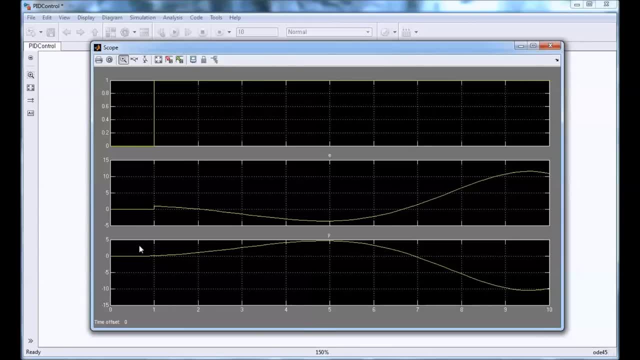 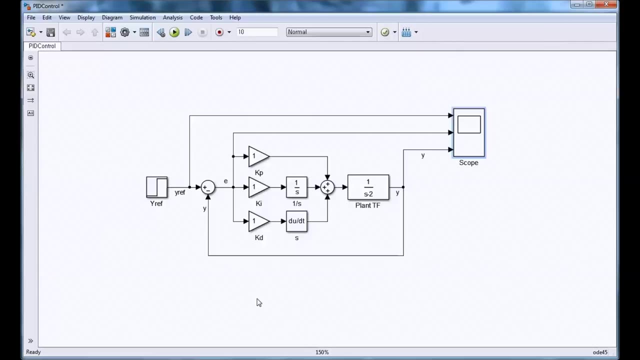 So we have our input coming in here, our Y ref. our error is going all over the place, and so is our value. So just putting a PID control doesn't necessarily work. You have to pick the right values. So for this one we wanted to make it exactly. 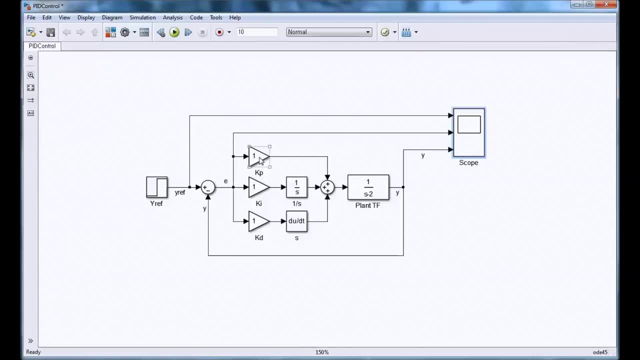 a negative one, negative one pole. So we have to now change our values. So if we look back at what we just derived, we found that KD had to be actually equal to zero, And what this means also is that we're actually not using the D part of this control, So it's actually just going to be. 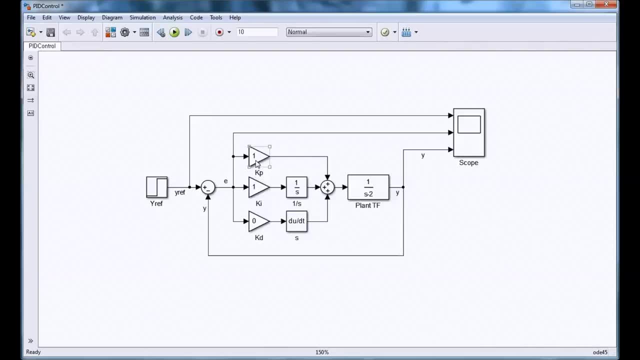 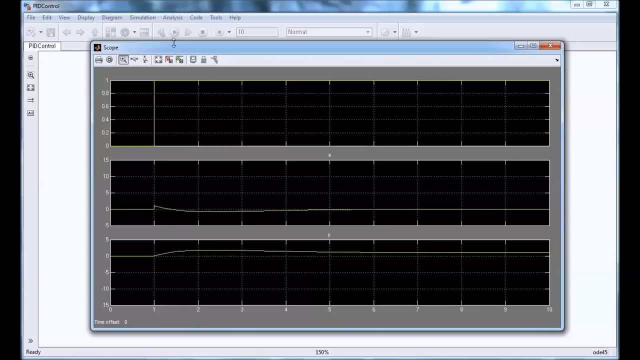 a PI control And our KP value here was four And our KI value was one actually. So we're good there. Let's see if just changing those values will make a difference in our system. So run it and let's look at our system. We see that.